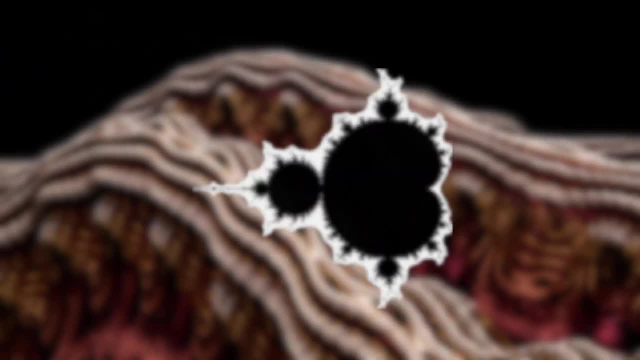 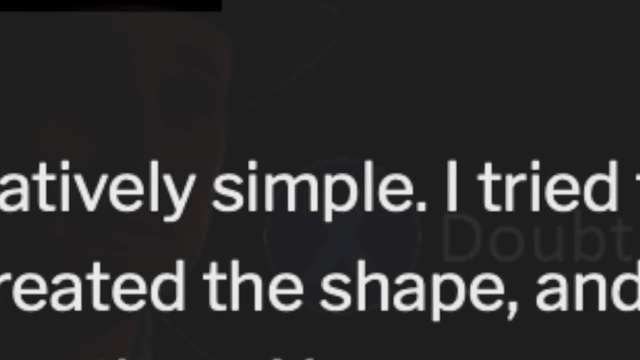 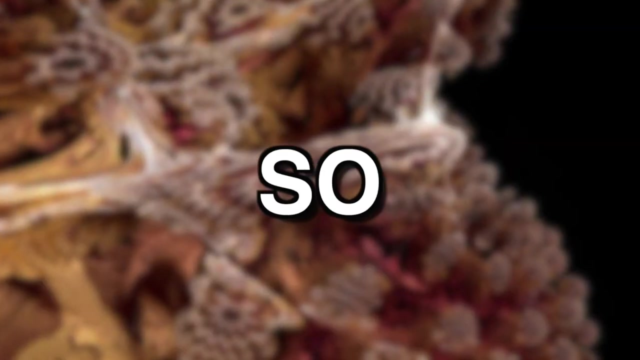 to 2007, a bloke called Daniel White wanted to find out if a 3D version exists. So Dan and a number of people from the fractal forums used some relatively simple maths and finally discovered the closest thing we can get to the 3D version: the Mandel bulb. So now let's look at how some other 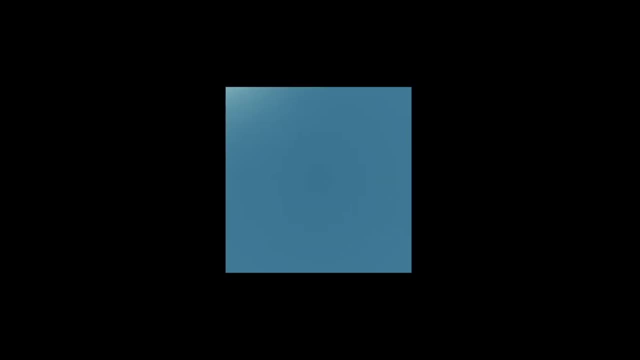 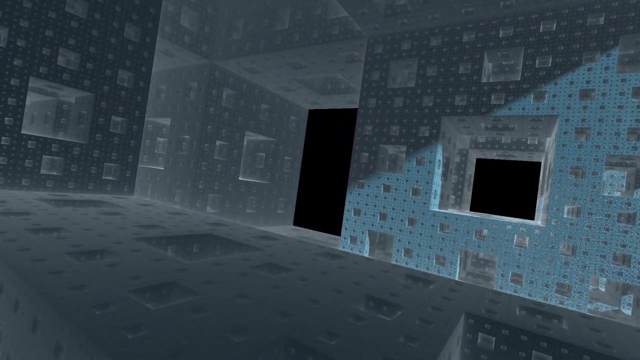 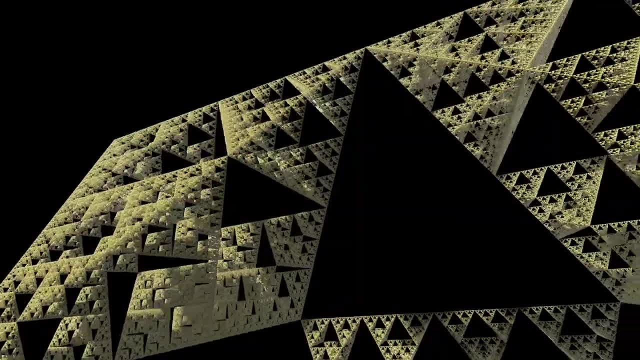 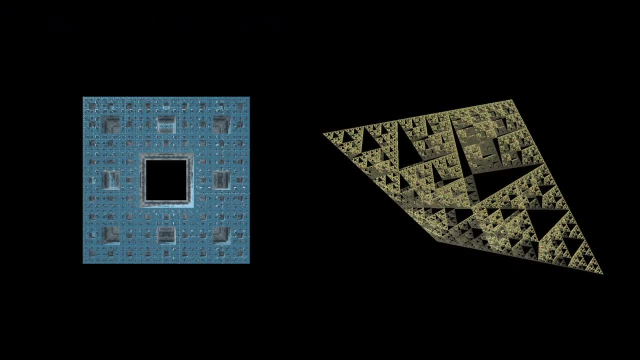 we made here is called a Menger sponge. We can do this with pretty much any shape we want. This one is called a Sapinski tetrahedron because it's made from tetrahedrons. Whilst these are already cool, you kind of know what to expect with them. So how do you make these super alien looking? 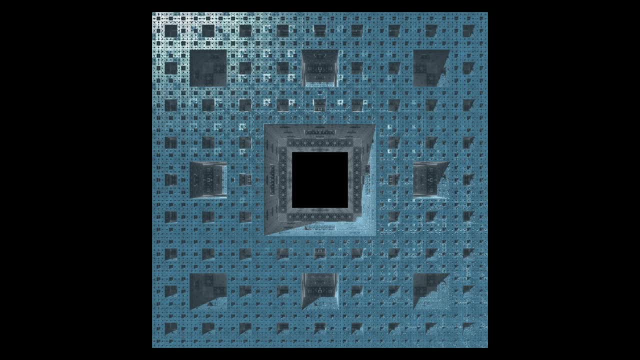 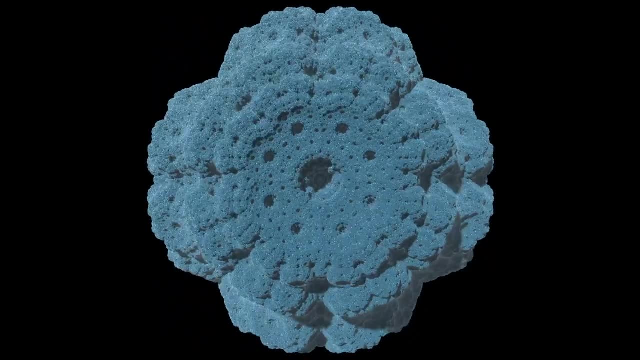 fractals. Let's start with the mandrel box that I showed you and use that as the base of our fractal. We can add a spherical fold, add an x-axis rotation, then add a z-axis rotation. All of a sudden we have something pretty complex looking And if I had NASA's supercomputer we could keep. 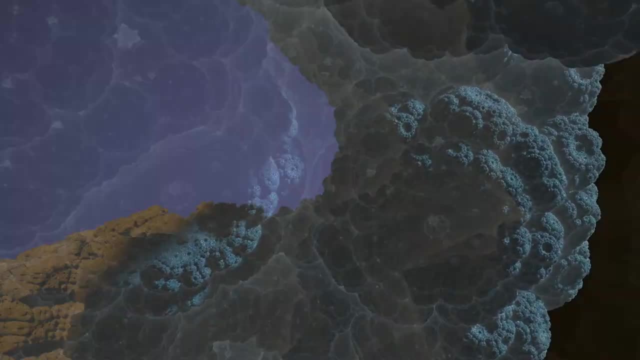 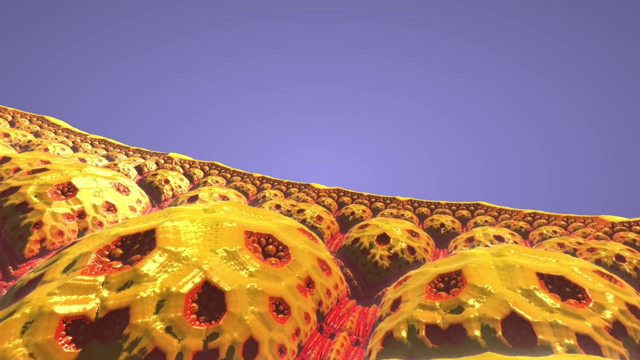 zooming into it for a long time and keep finding detail. We can also morph the fractals in real time as we're flying around them. So how is this massive amount of detail possible to render while still keeping a reasonable frame rate? For that we have to explore the technique used to render. 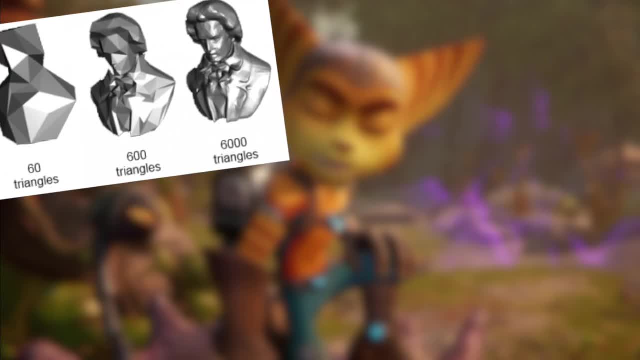 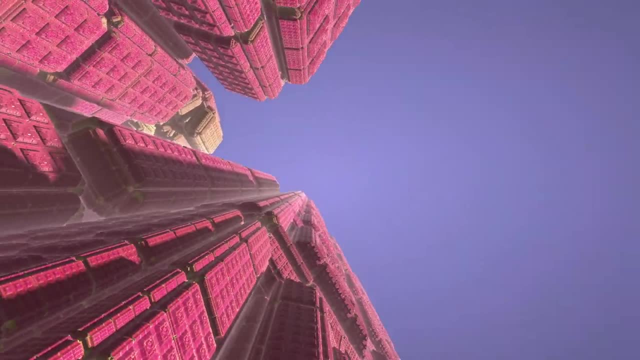 them. You're probably aware that most games use many different triangles to render a whole object. This is called rasterization. Because of the amount of detail in 3D fractals, it would be unreasonable to have to render that many triangles, And you don't want someone. 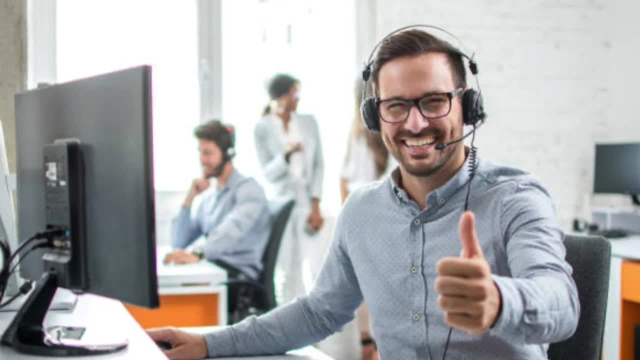 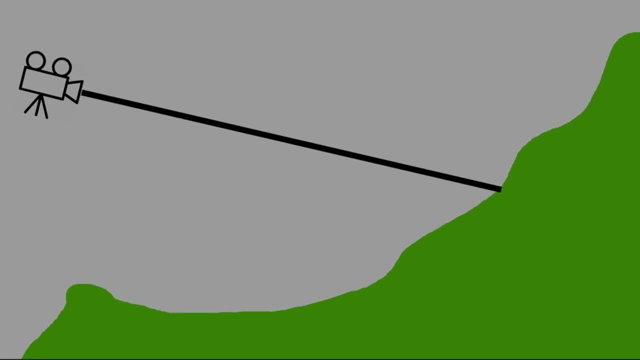 sitting there just modeling the same thing over and over forever. They rendered using something completely different, called ray marching. First we cast a ray out from the camera. We check for objects to draw by drawing an imaginary circle around the ray As we get closer to an object. 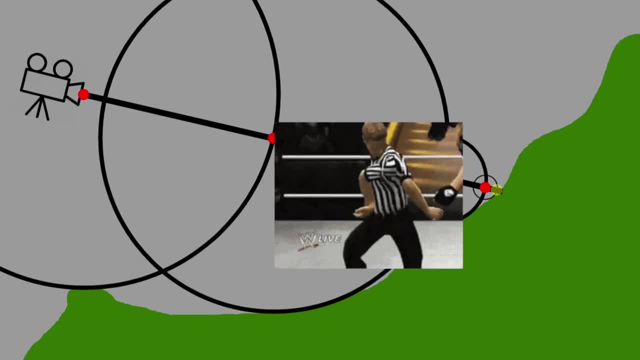 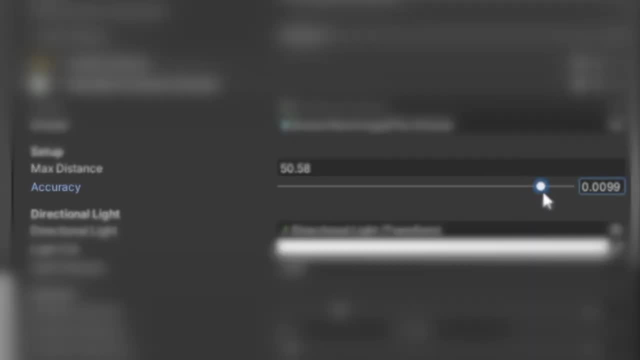 the circle gets smaller. When it gets smaller than some distance we define, it draws the object. This is done many times until the whole object is drawn. As we make the threshold for the circle lower and lower, the fractals become more and more detailed, until some point where it slows. 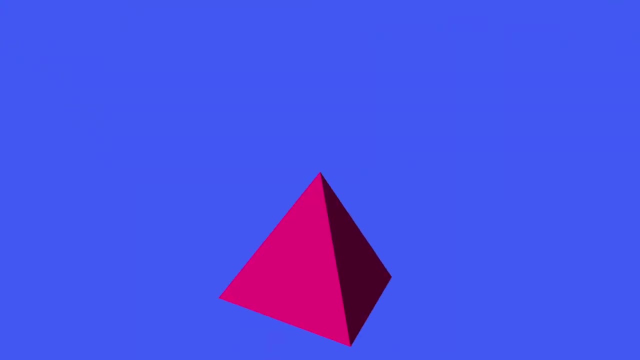 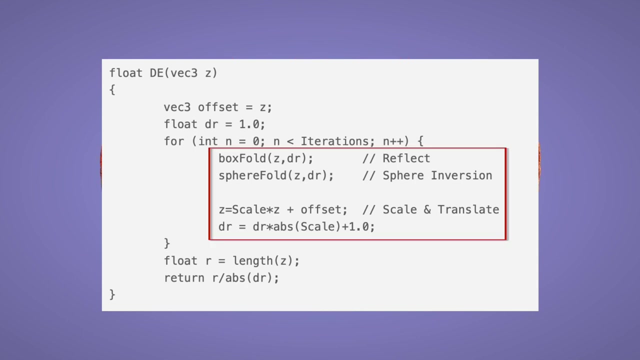 down so much that it We can tell the ray marcher the shapes to draw using something called a distance function. This is what makes ray marching so good for rendering fractals: We can just tell it to follow some rules and to repeat them over and over, No triangles necessary. 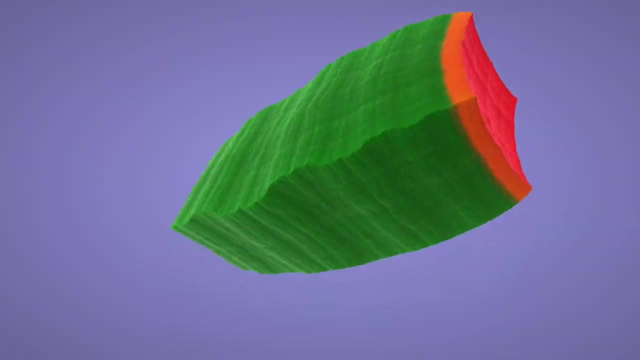 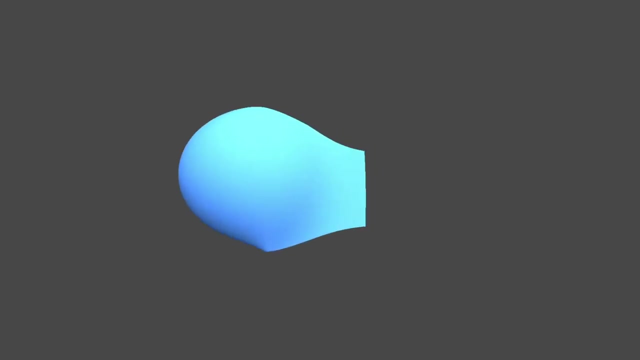 Because of how different it is from rasterization. ray marching has a bunch of other cool it can do at basically no performance cost, like render an infinite amount of a shape and blend shapes together. Even with ray marching trying to increase the detail too much, still makes the 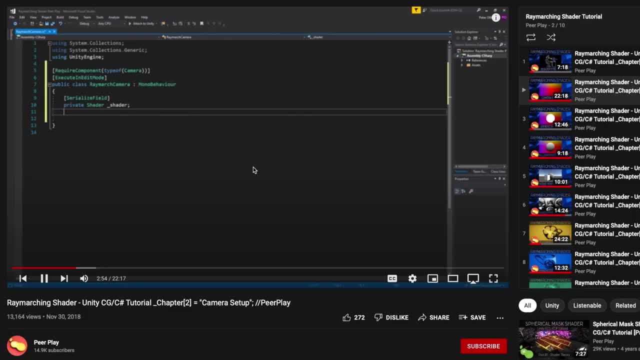 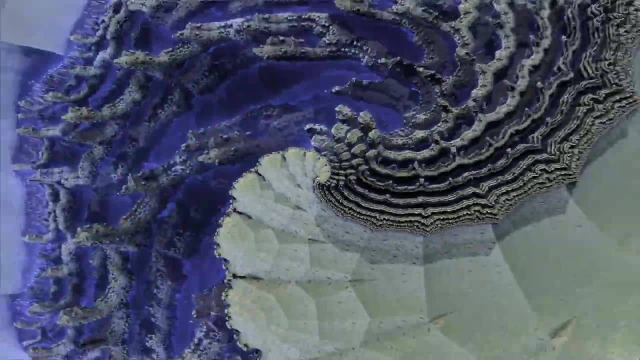 FPS go to hell? I was asking myself this question when I was building my own renderer for these. So let's create a public material. I saw these amazing looking renderings that seemed to go on forever and I was wondering how I could make them myself, Because you know. 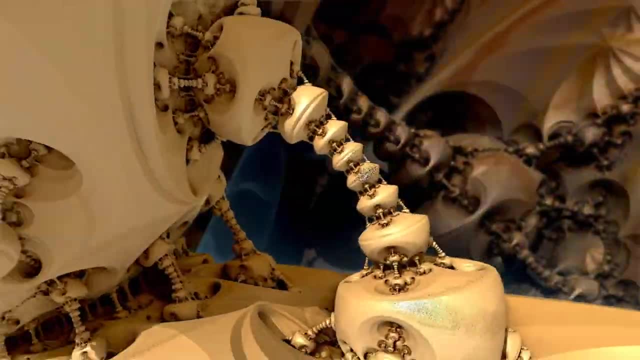 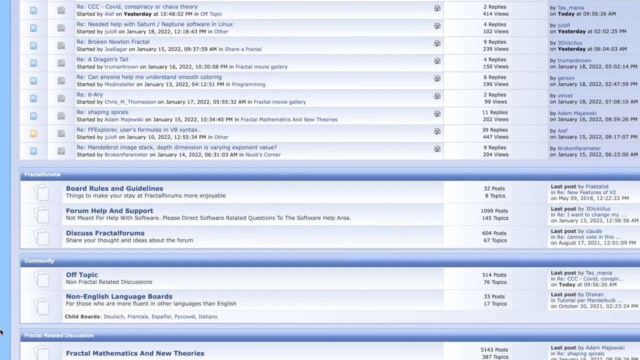 After some googling, I found out that these super complex animations can actually take weeks to render. That's when I stumbled upon the fractal forums which I mentioned at the beginning of the video. It's literally a whole community dedicated to talking about these things and making them. 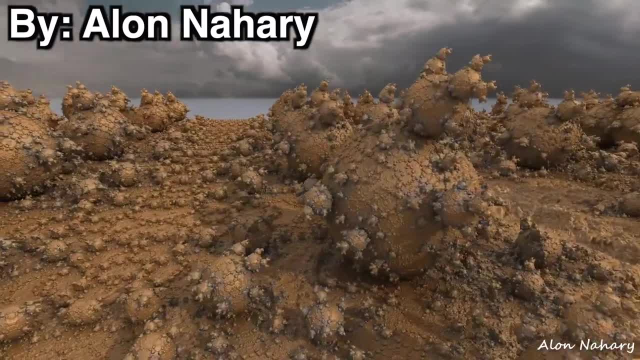 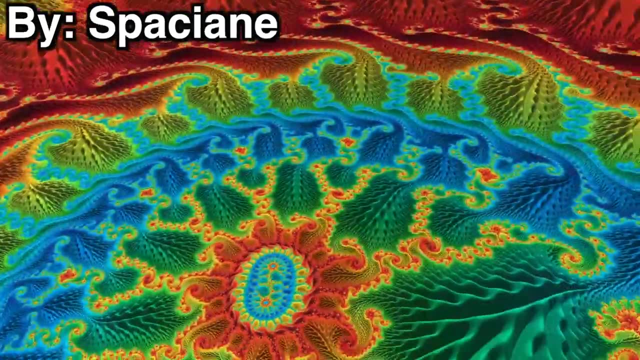 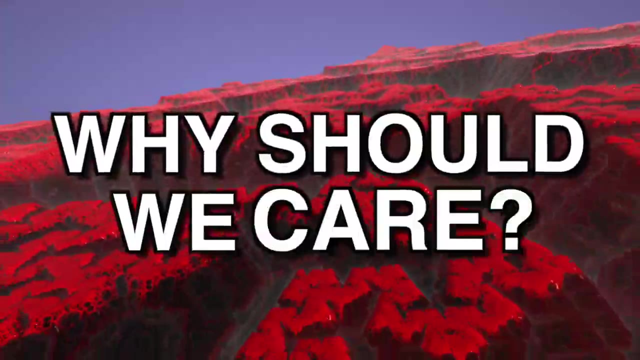 Let's look at some creations of the members. So this all looks really cool, but why should we care about these in the first place? Well, it turns out fractals have a lot to do with nature On a small scale. it's a very simple idea, but it's also a really cool idea to think about. 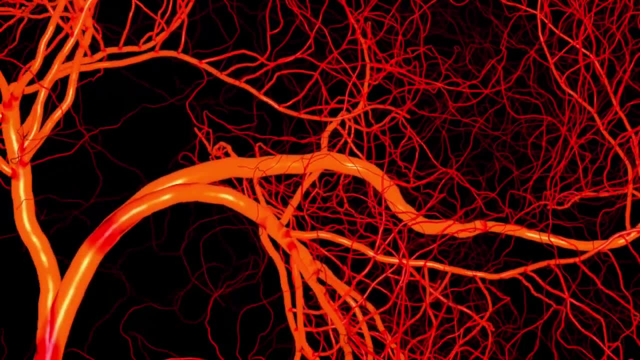 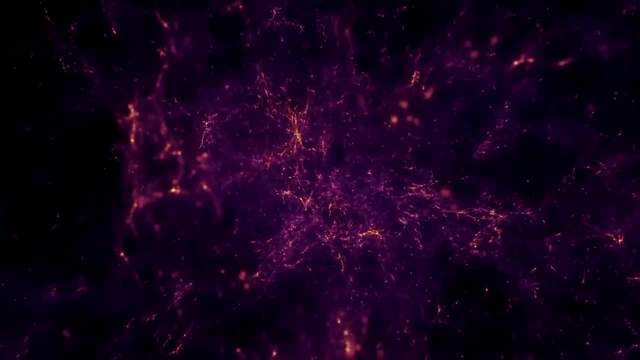 It's a really cool idea to think about. but it's also a really cool idea to think about On a larger scale: trees, cauliflower, our own body At a bigger scale, solar systems, galaxies, even our universe at its biggest scale kind of looks like a fractal. We subconsciously see them. 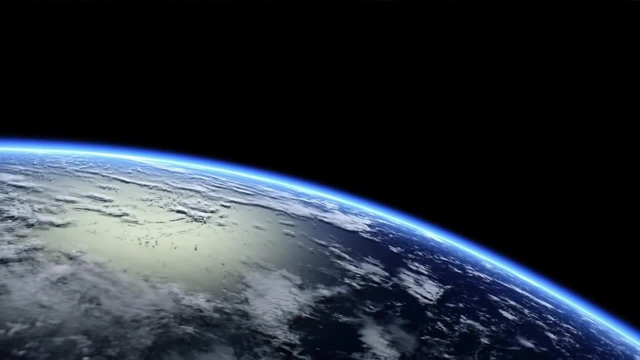 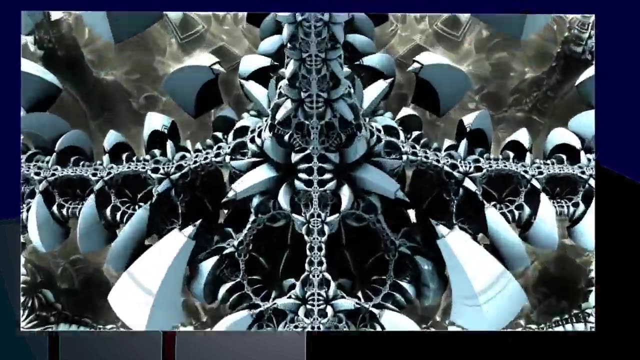 everywhere. It's a glimpse we can get into infinity. Born too late to explore the world, too early to explore space, but just in time to stare into your monitor for hours looking at fractals If you're interested in making and exploring these yourself.